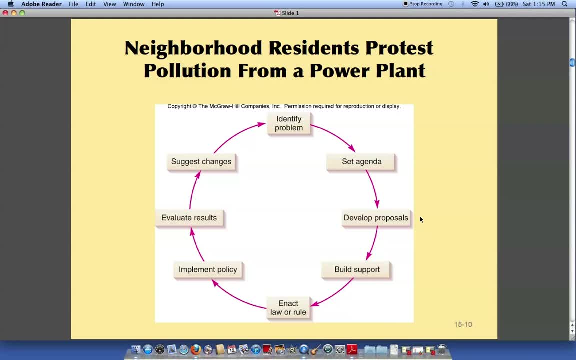 And That would be the hypothesis. And then they create rules and they implement. Would there be experimental and data? And then they evaluate. That would be their conclusion. They're evaluating their policy And then they redo it, rewrite it. 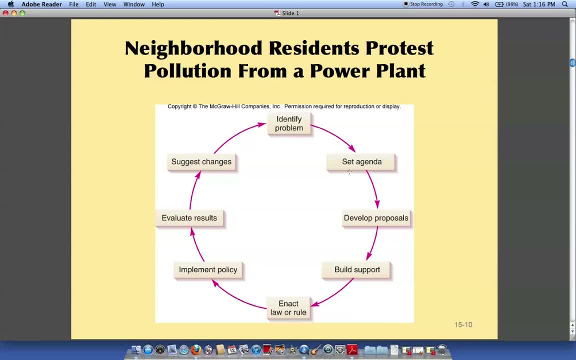 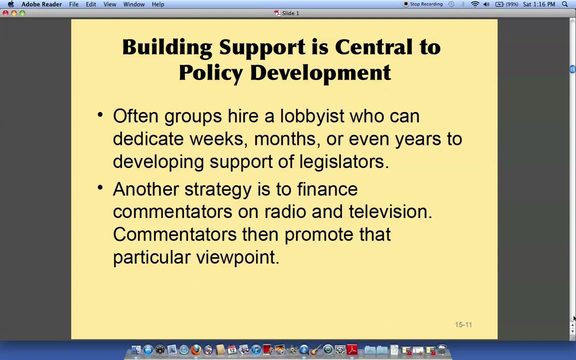 And then they go about correcting their policy. So it's kind of like the scientific method in our problem solving. So of course support is always needed. when you want to get into the policy making, You need to have support of the citizens, Then you need to get support of your city. 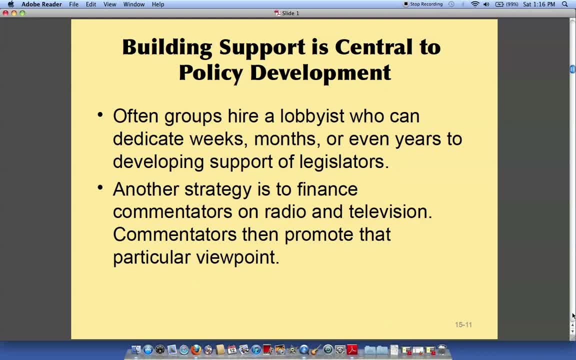 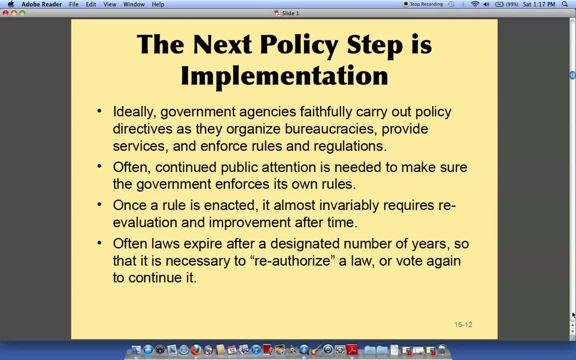 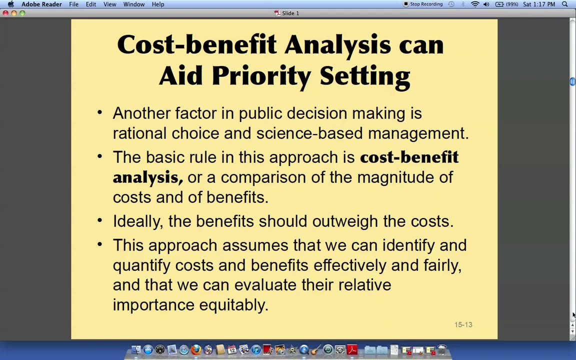 or county County commissioners and all of this. it then goes up to the senators and so forth. Then the government has to approve it And then you can put it to a vote, And then there are some cost benefit analysis that are done. 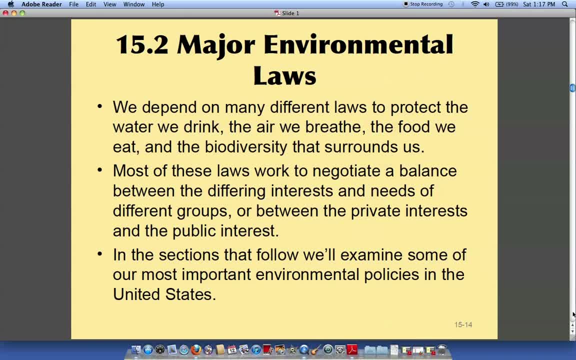 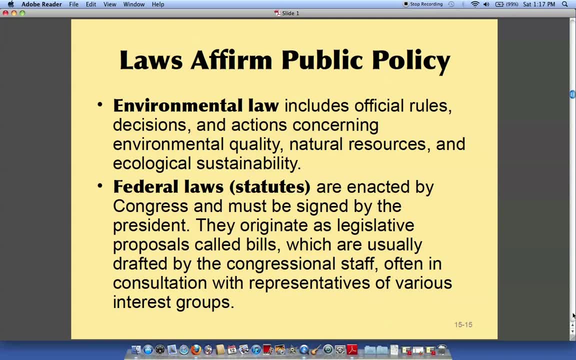 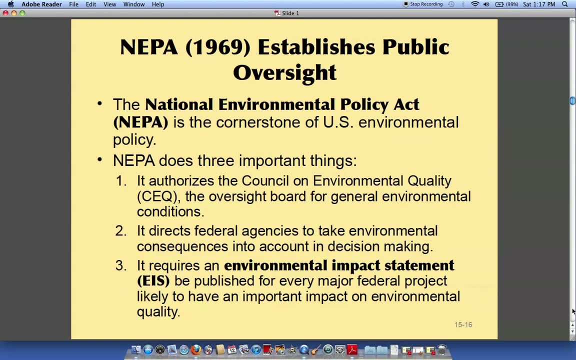 And then And then You know, some major environmental laws are created. I think you can read through this in your book and get more information from this: Our NEPA, National EPA. Most people know the EPA. I don't know if you know the EPA. 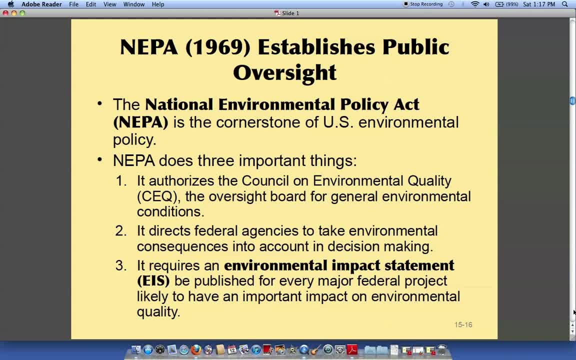 I don't know if you know the EPA. I don't know if you know the EPA- Most people know the EPA- Environmental Protection Agency- But this is the National Environmental Policy Act. okay, So there are different things there. So all of these policies require impact statements. 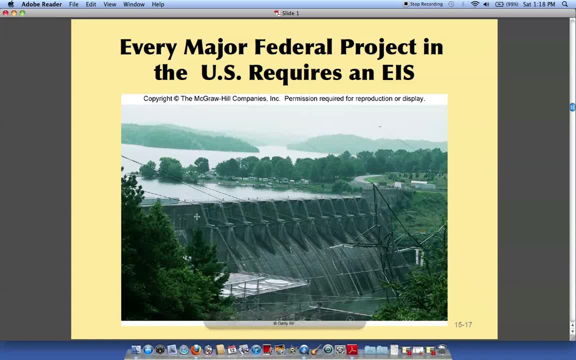 How would this dam, for instance, impact this a dam, this environment? How is this going to impact the fish, the other organisms, the plants and other animals that live and need this area? before this dam was built, You know what's going to be affected. 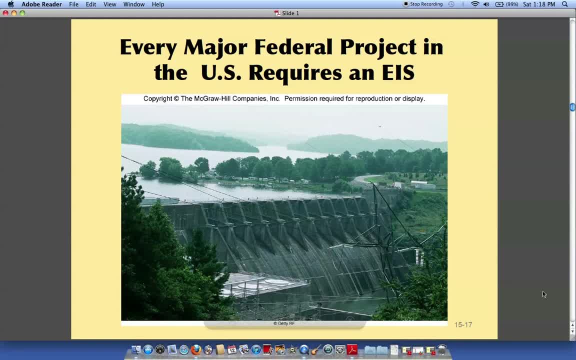 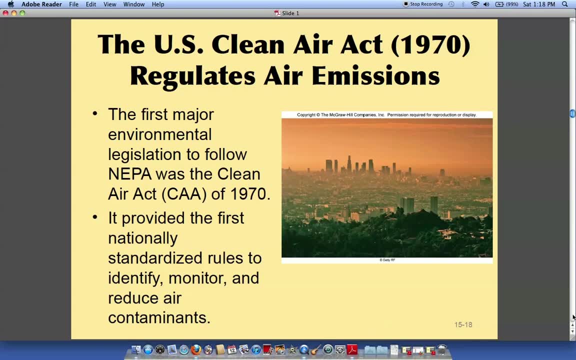 An environmental impact statement. okay, And here's another one. The Clean Air Act regulates emissions. Well, I think they need to require some of these polluters to clean up their act. We have a lot of factories and things that have extensions on their policies of cleaning up their smokestacks. 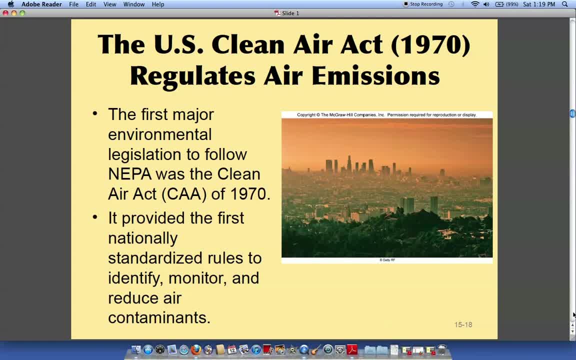 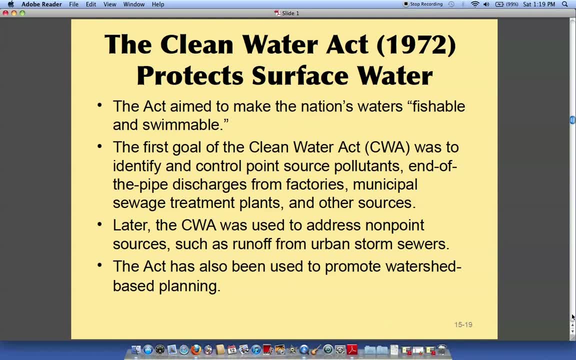 and I think we need to buckle down, because we do have our global warming going on here, Our Clean Water Act- this is very important. However, certain petroleum companies are now searching for basically leftover fuel and petroleum, And the reason why we're looking for these is 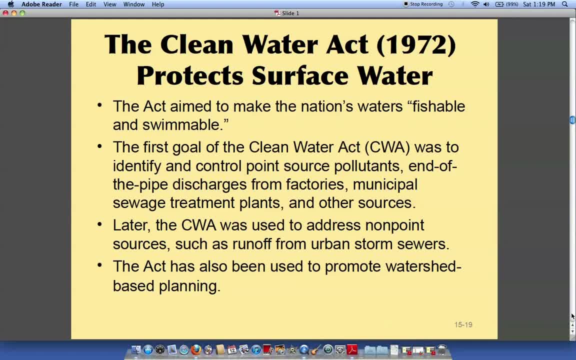 because they're looking for petroleum in the petroleum industry. Petroleum industry is an area that's very important, And they're trying to do that by using petroleum in, by using a method called fracking, And this is that they force water down into these cracks and crevices. 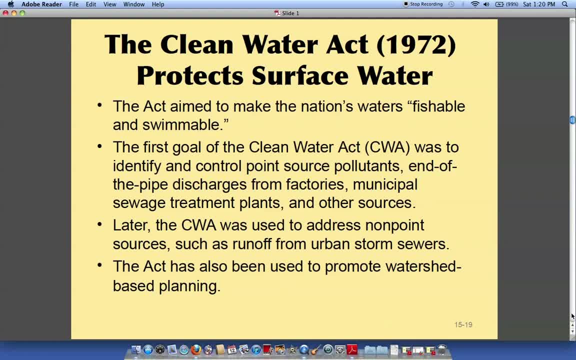 And that pushes these petroleum products up to where these companies, these oil drill companies, petroleum products. then they can suck it out. but what happens if these methods actually put petroleum in our drinking water? and a lot of people have wells in these areas and a lot of companies are just not even considering polluting. 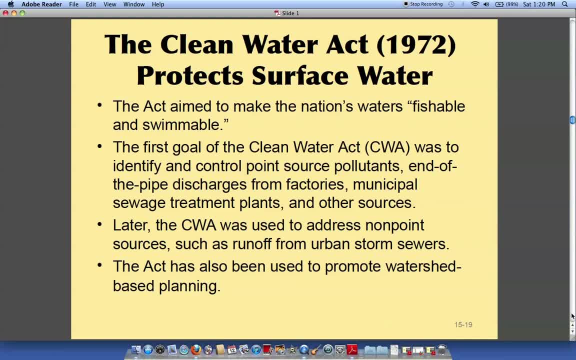 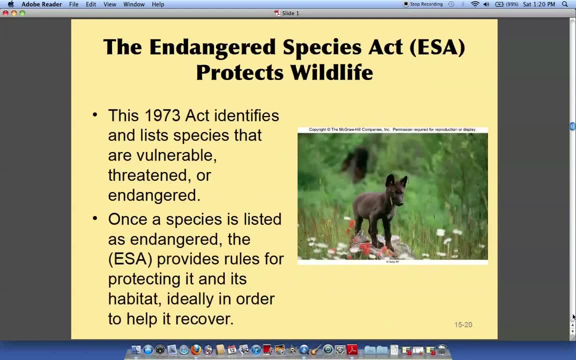 people's well water. so the attitude is: well, we'll try to fix it when it happens. well, that's not a good idea. so the Endangered Species Act- this is- has protected many species that have become endangered because of habitat destruction or other things that that have happened. mainly human humans are. 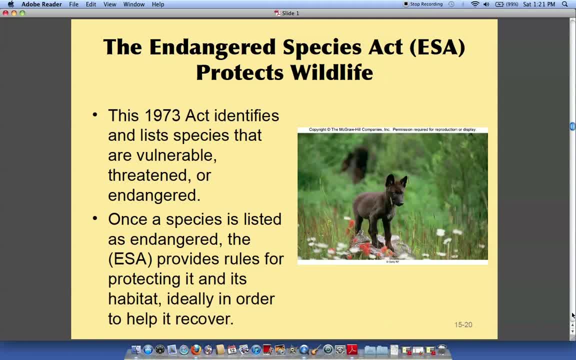 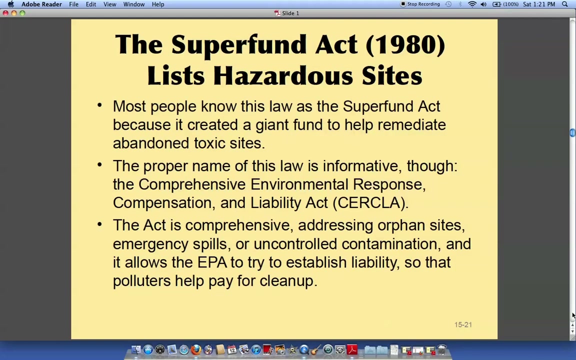 the cause, but we see that everything needs to be protected. our environment is very, very. the environment is the only one we have and we have to protect it. there are a lot of resources that we we really need to be careful how we manage them. we have superfund. 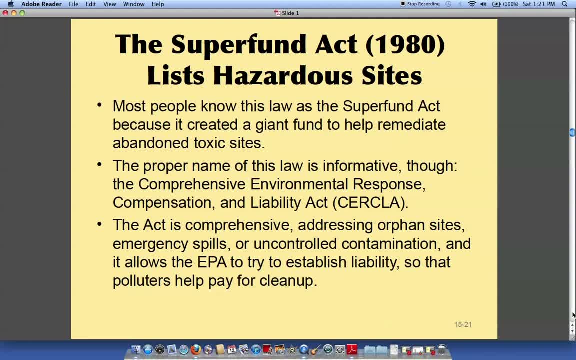 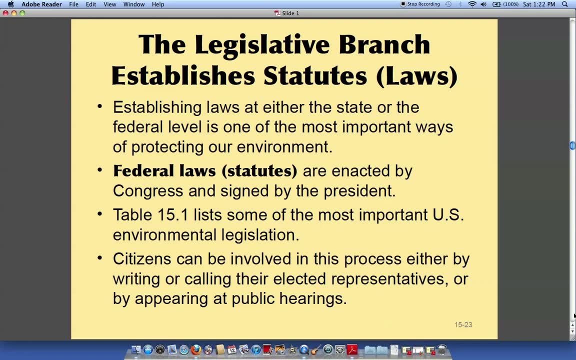 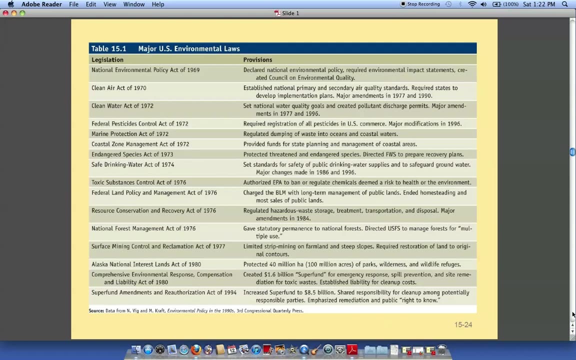 sites now that we have to dig up companies that have buried their hazardous waste. This is a big problem, And this next section talks about how policies are made and what kind of governmental branches make these policies. Here are some of the US laws, but these are US laws. 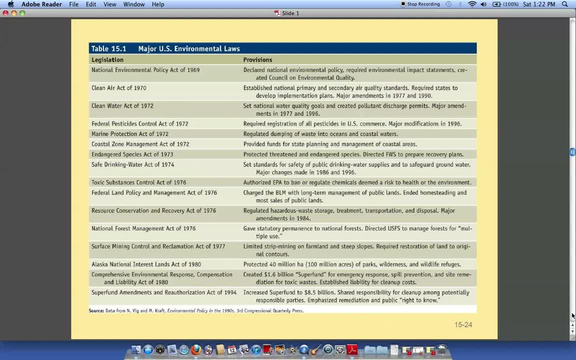 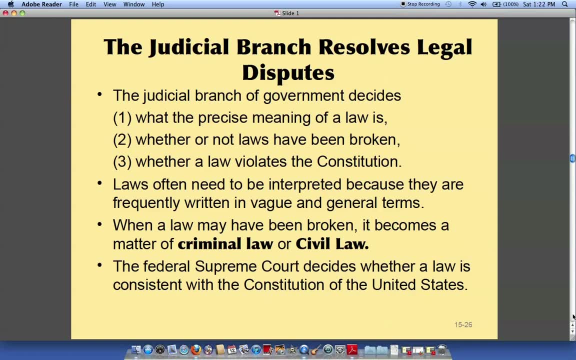 It doesn't mean that they are worldwide and environmental problems are worldwide. Criminal law, there's environmental law. This is you know. if you're thinking about being a lawyer, you might want to go into environmental law. What happens when people break the environmental laws? 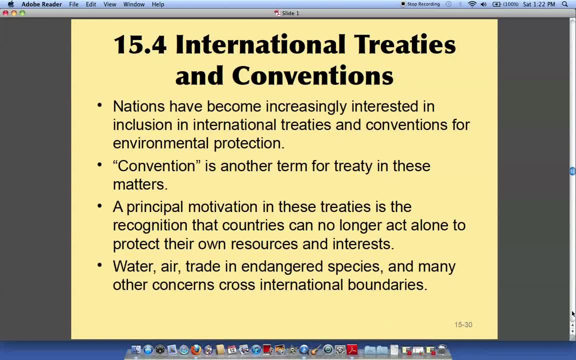 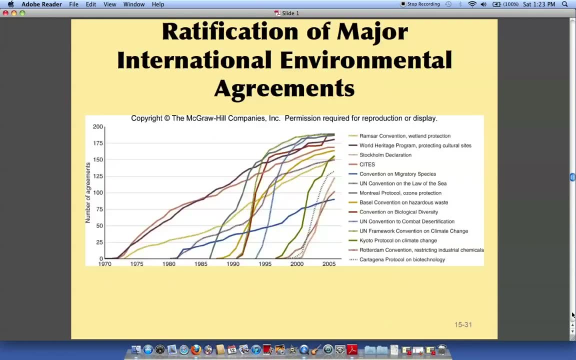 Okay, We have. We have to try to work with other countries to help conserve the environment, And so we get together and we discuss things and hopefully, you know, other countries agree with us that we need to save these resources, these valuable resources. 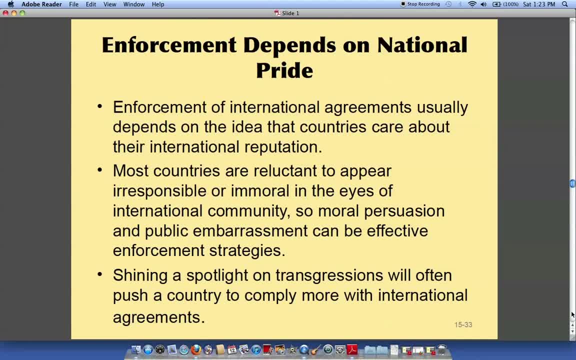 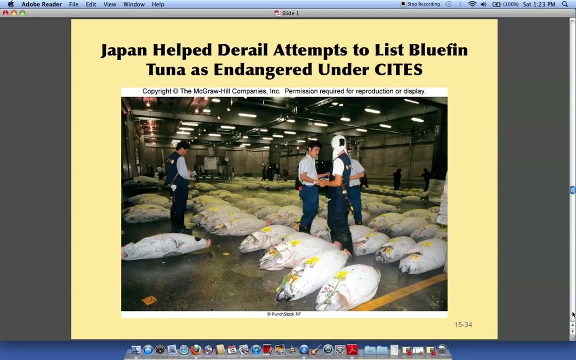 and manage them properly. Sometimes, getting nations to adhere to environmental conservation, we might have to embarrass them to do that, but somebody's got to protect the environment. This is what Japan does with the tuna is horrible, and it's They're exploiting the tuna. 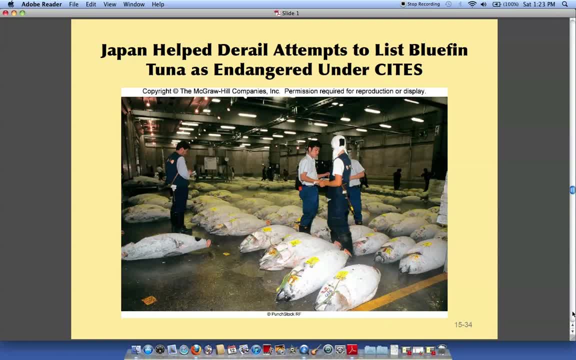 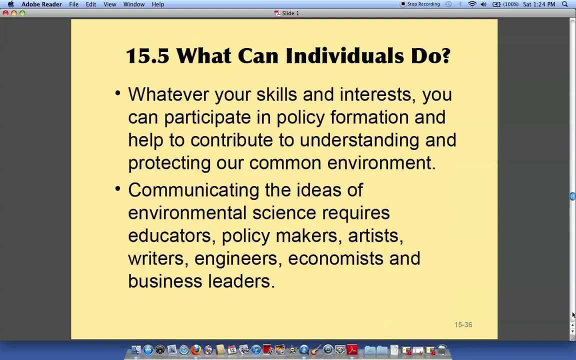 and this is another one of our fish industries that is going to tank. if countries that exploit them, exploit the tuna, do not stop, We just may not see tuna in our future. What can we do? Well, all we can do is what we can do, you know. 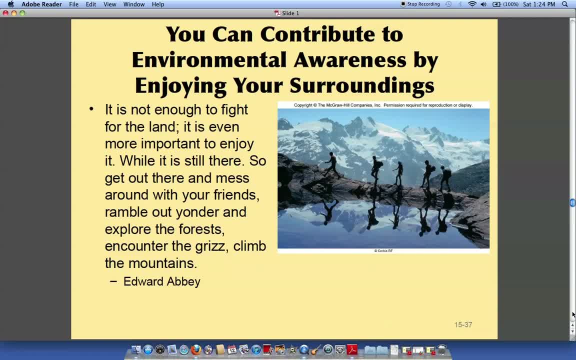 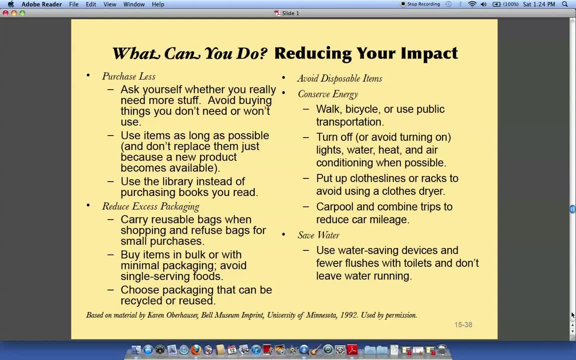 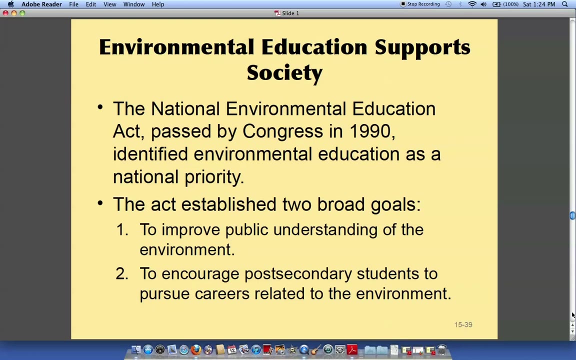 You either become an environmentalist or you donate to environmental groups that actually go out and help. Some simple things you can do. So this is just an overview of a few things you can do As a single person. get your family involved. 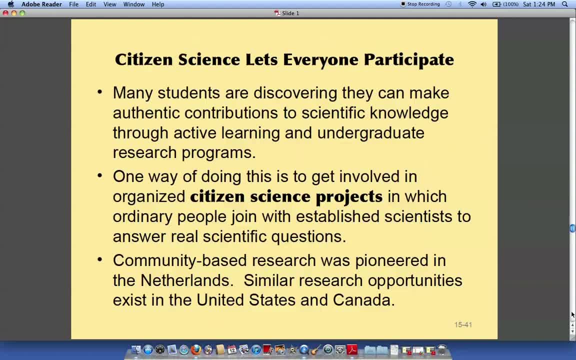 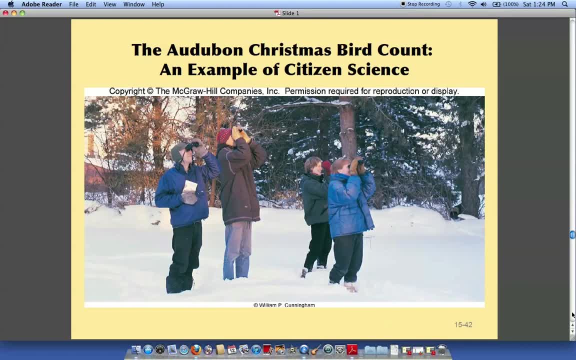 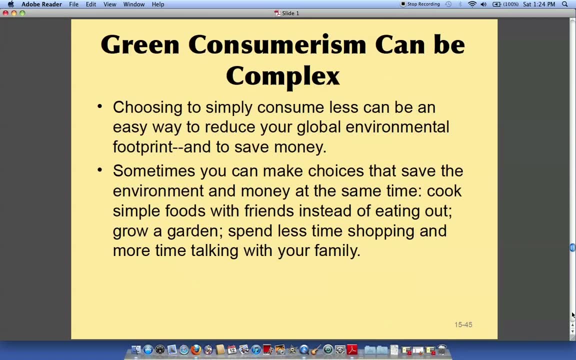 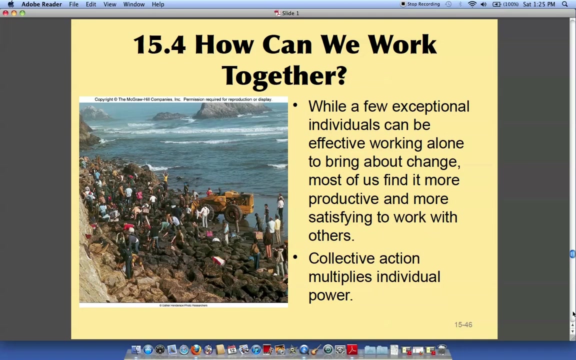 Go out and become aware of your natural environment. Okay, Participate in bird counts. I've done several of those. How much do we really need? You can try to be green by stop using those plastic bags and reduce your footprint. Help on a cleanup or a planting. 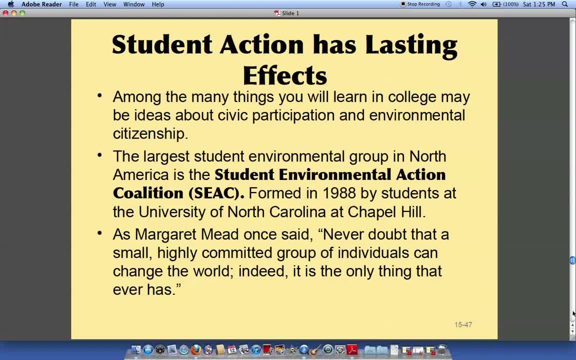 Go out and help the community Student Coalition. You can go online and check out and see if there's a student group. at our college We have the Biology group that gets together and helps to do a few events to help clean up the environment.